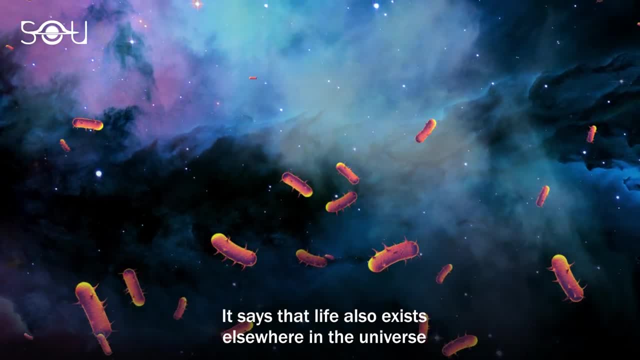 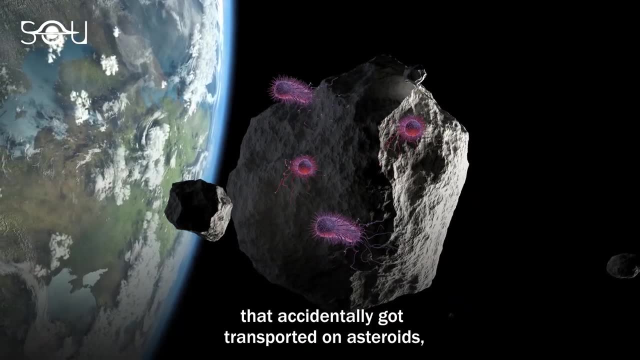 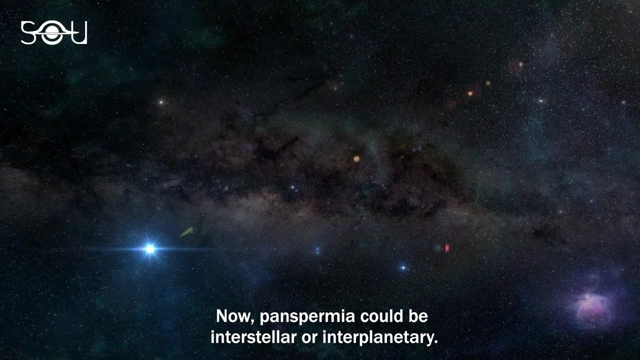 word panspermia means seeds everywhere. It says that life also exists elsewhere in the universe due to a distribution of microorganisms that accidentally got transported on asteroids, other traveling planetoids or even spacecraft. Now panspermia could be interstellar or 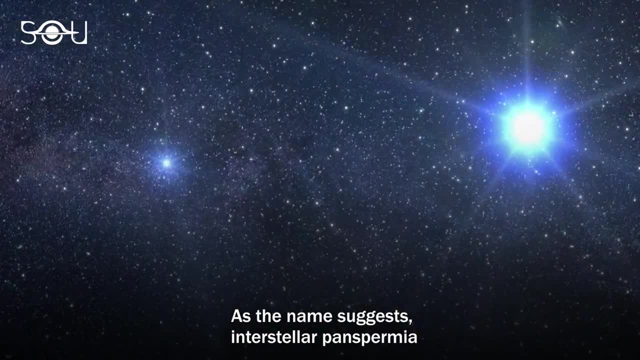 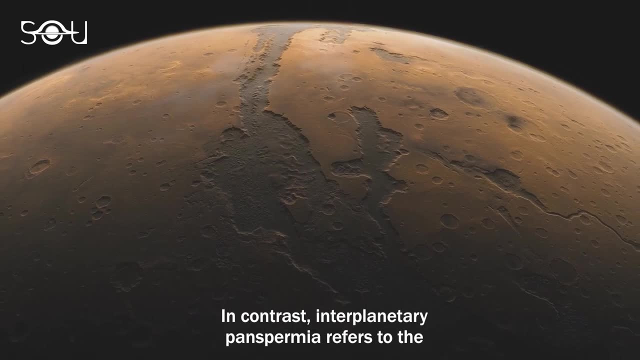 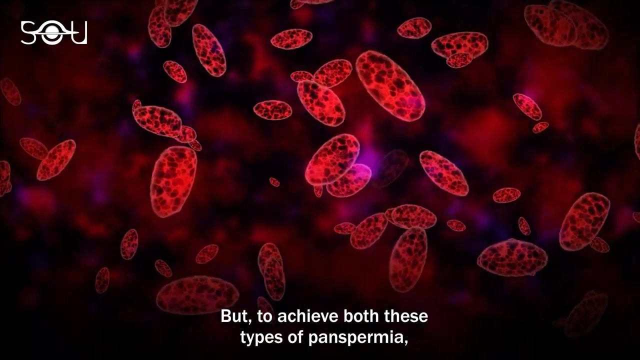 interplanetary. As the name suggests, interstellar panspermia points at the transportation of life between different star systems. In contrast, interplanetary panspermia refers to the transport of life from the neighboring planets and stars. But to achieve both these types of 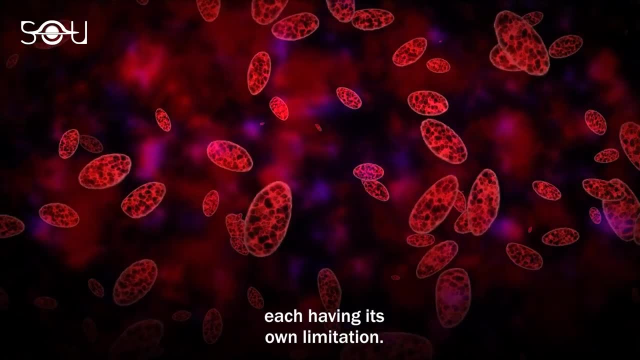 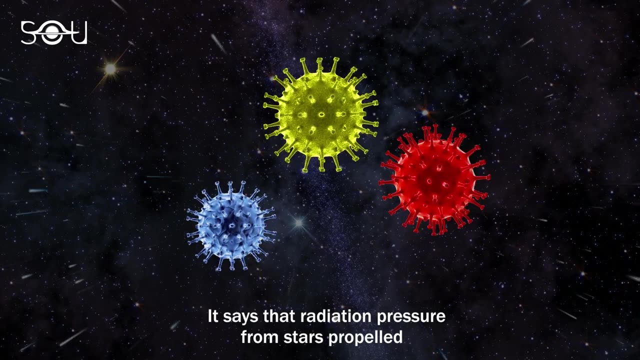 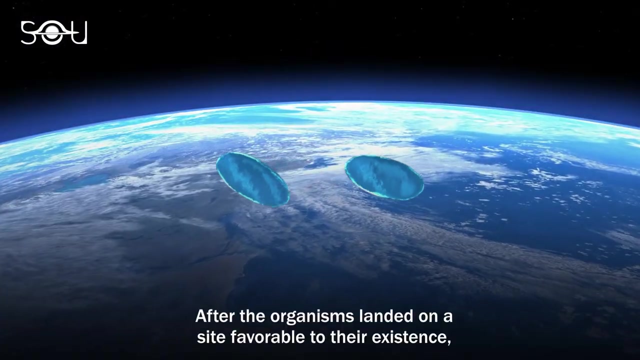 panspermia, three mechanisms have been proposed, each having its own limitation. Let us begin with radiopanspermia. It says that radiation pressure from stars propelled microorganisms through space until they reached an object to land upon, After the organisms landed on a site favorable to their 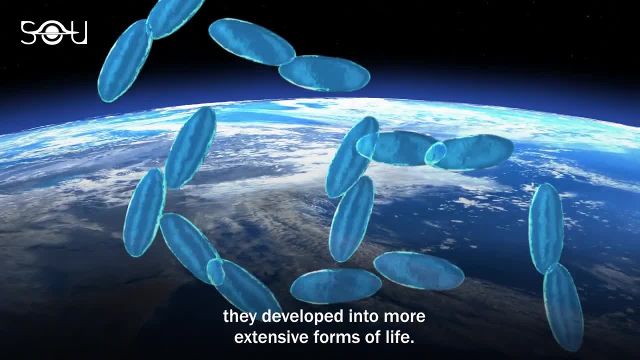 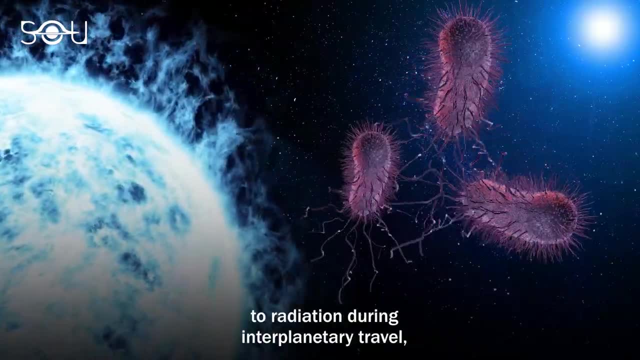 existence, they developed into more extensive forms of life. But radiopanspermia is not the only way to achieve this. There are other mechanisms that can be used to reduce the chances of successful radiopanspermia, Due to the long exposure of bacteria to radiation. 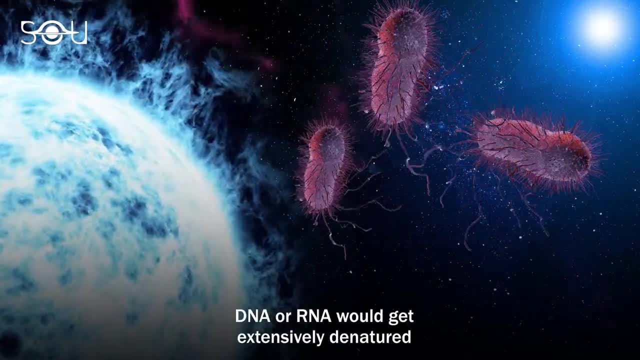 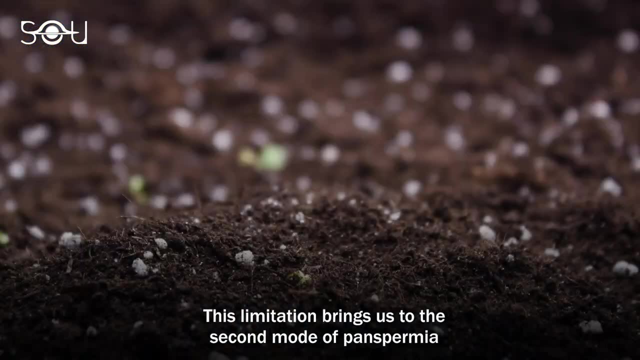 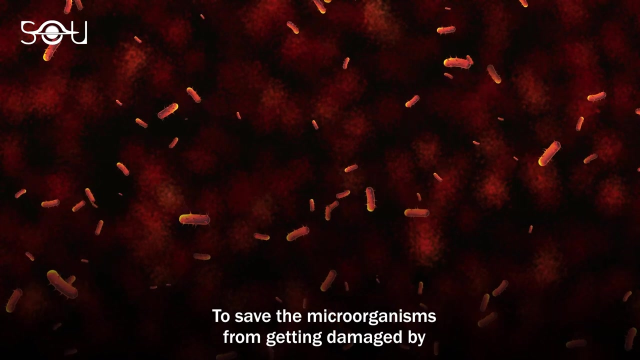 during interplanetary travel, DNA or RNA would get extensively denatured and reduce any chances of successful radiopanspermia to almost zero. This limitation brings us to the second mode of panspermia, which is lithopanspermia, To save the microorganisms from getting damaged by harmful 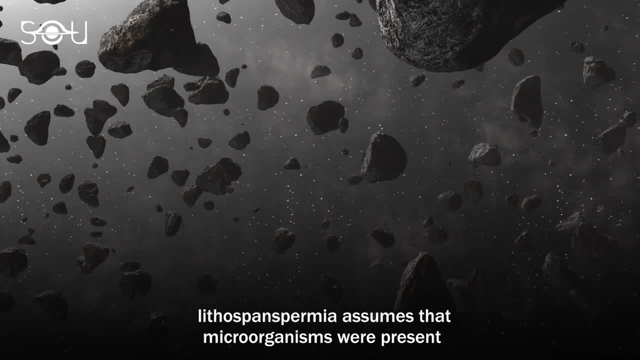 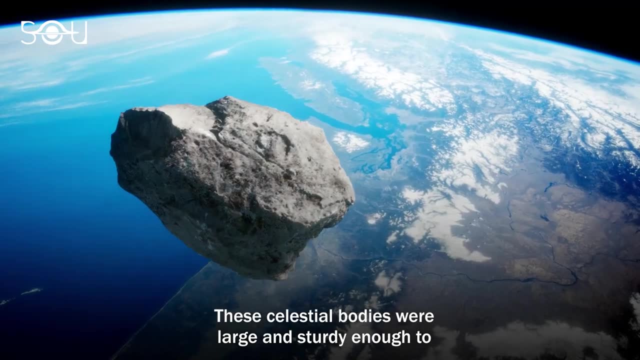 cosmic radiations. lithopanspermia assumes that microorganisms were present on or in asteroids, comets and other planetoids. These celestial bodies were large and sturdy enough to withstand planetary ejections, lengthy travels along with powerful atmospheric re-entry, thereby carrying 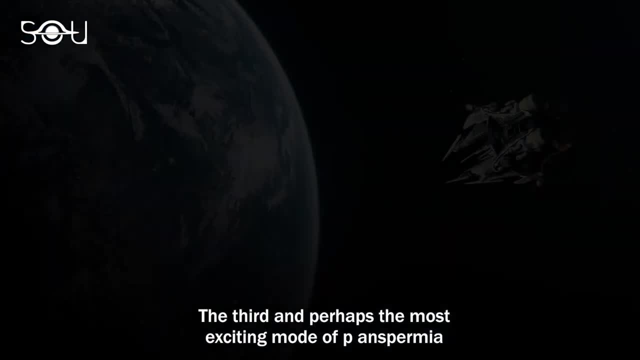 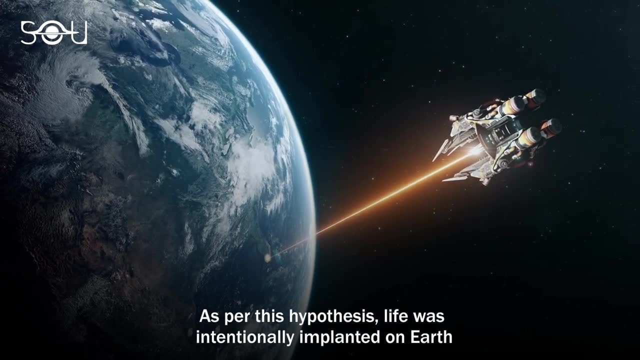 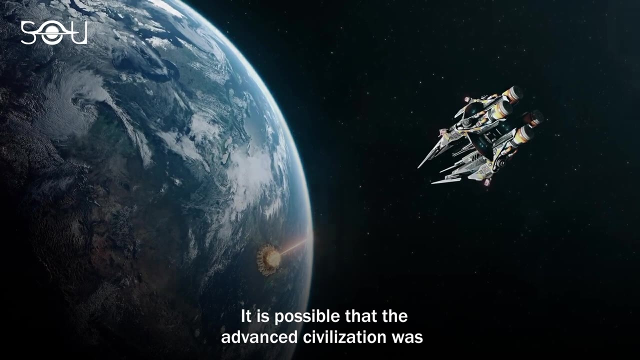 out safe transportation of life. The third, and perhaps the most exciting mode of panspermia is intentional panspermia. As per this hypothesis, life was intentionally implanted on Earth by an advanced extraterrestrial civilization, or maybe it was merely an accident. It is possible that the 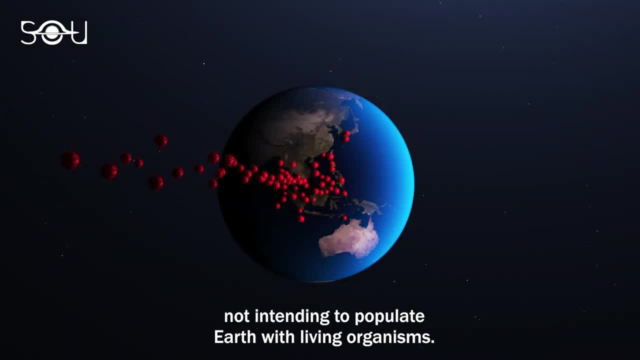 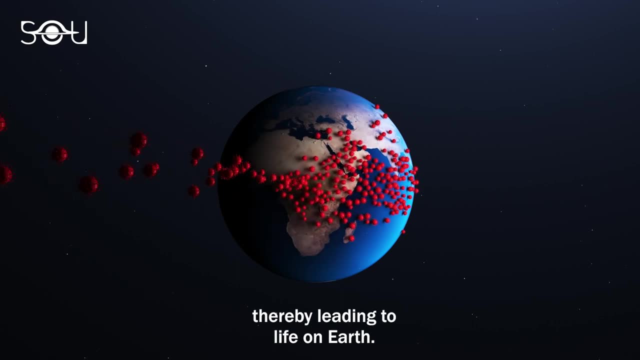 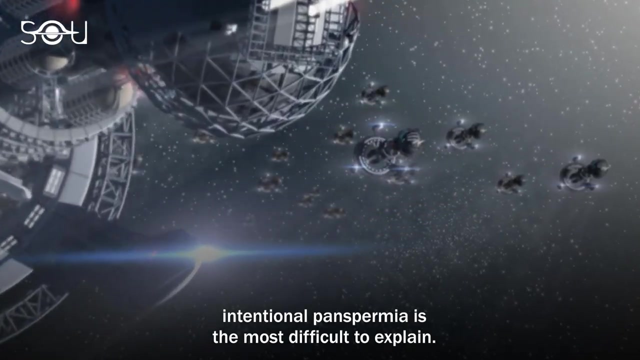 advanced civilization was not intending to populate Earth with living organisms. Instead, it was only disposing of its organic waste that accidentally landed on planet Earth, thereby leading to life on Earth. Given that we haven't found any intelligent civilization in space, intentional panspermia is the most difficult to explain. After all this, you may be wondering if the